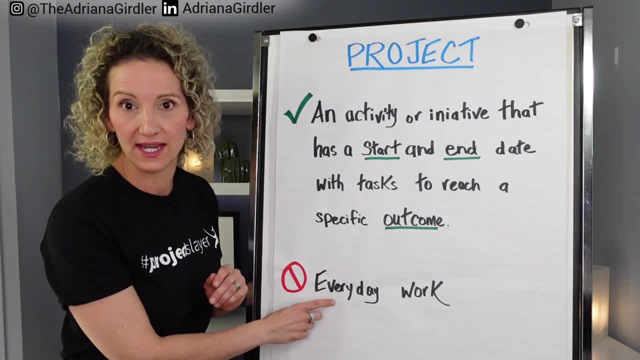 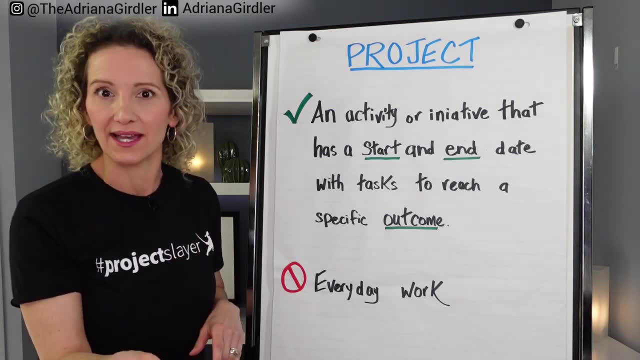 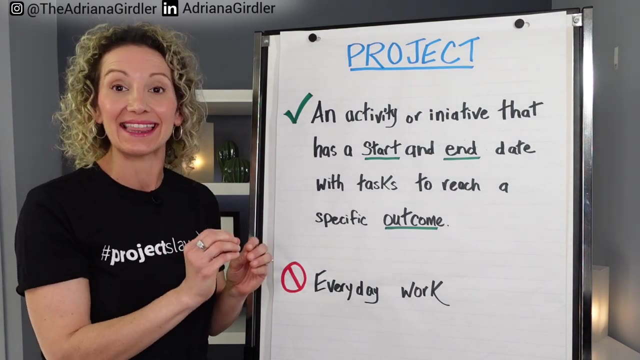 I want to be really clear. Projects are not everyday work. So if you have a task that you're repeating constantly over and over, that's not a project, That's an everyday work task. So just note this whole start and end date is really key- the temporary in nature, to indicate that at the 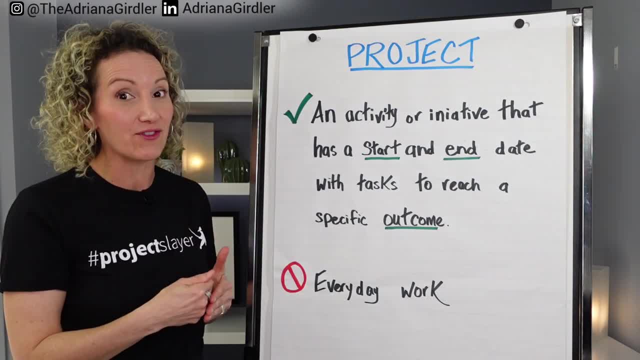 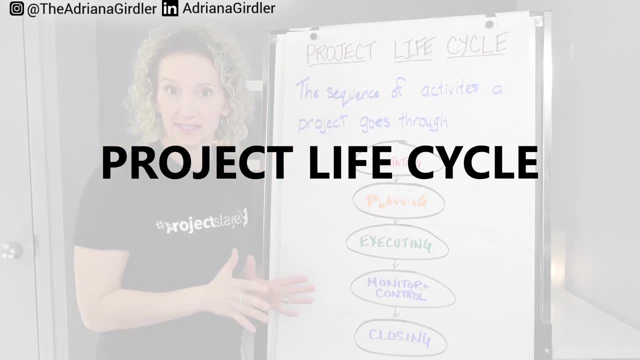 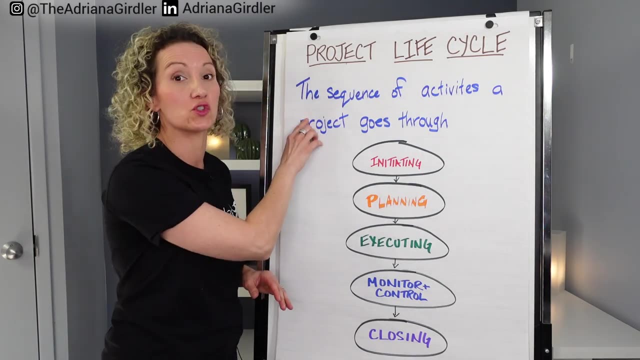 end you have a specific deliverable that you did not have when you started, but you now have it at the end. That's a project Project life cycle. This is going to be one of the most critical project terminologies you really need to understand, because all projects go through this life cycle. So 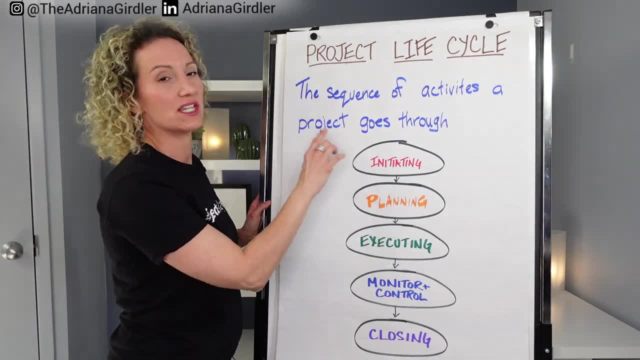 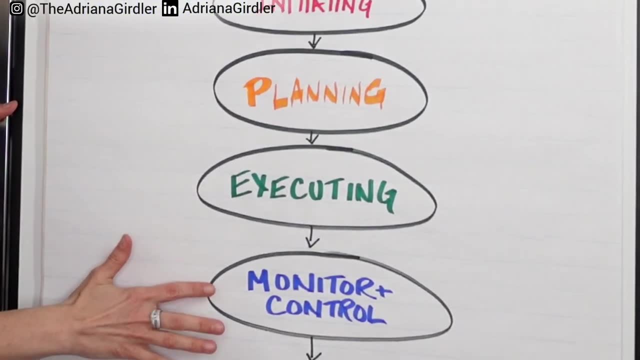 let's just get to the definition so you understand it more. It's a sequence of activities that a project goes through, and there's five distinct phases. There's initiation, planning, execution, monitoring, control and closing. Now what's really cool is it doesn't. 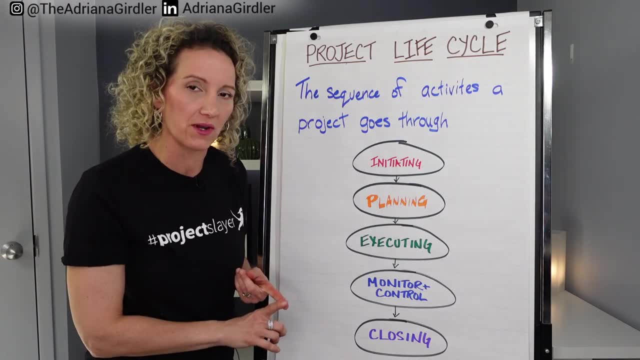 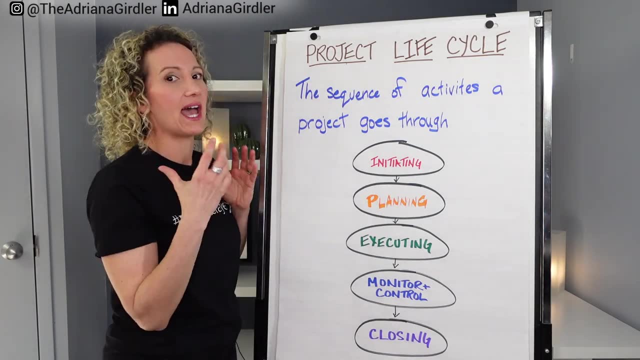 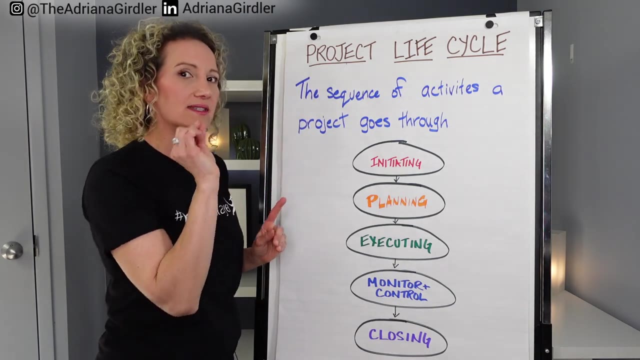 matter the project methodology you use, whether it's a waterfall methodology, an agile methodology, hybrid methodology, whatever it may be, they all go through this stage, And so if you have that fundamental understanding this is the framework of projects, then you'll totally get it. So let's just go one step further, because just the definition is great. 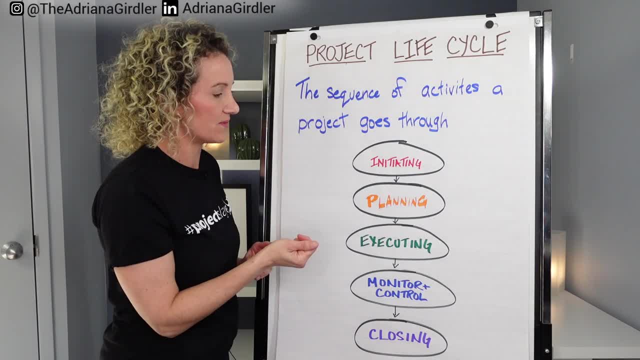 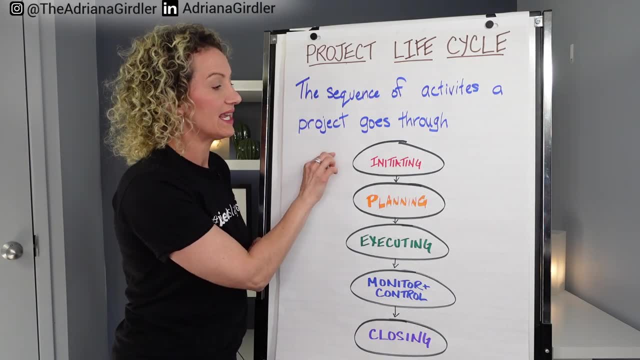 and I'm glad you have it now, but I want you to have a little bit more understanding of it. So a lot of people think projects are all about execution, and it's not. That's why this framework is important. It's really about initiating it, then doing the planning around it, getting all your 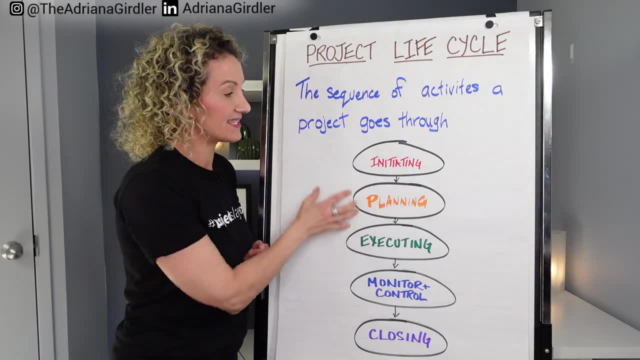 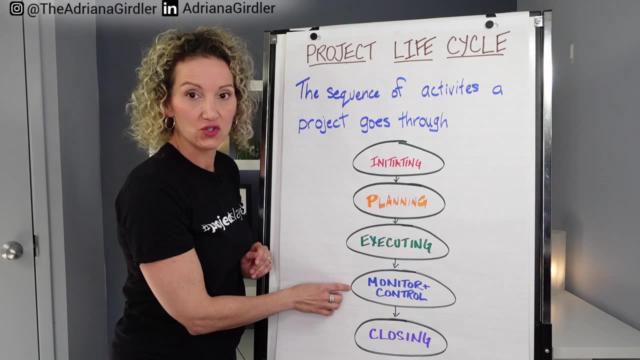 key pieces of information. The executing part is then taking what you've done over here with your team and your kickoffs and your sponsors, and you execute it, And then with the monitoring control. what's really cool and what people don't understand and realize is that there's an 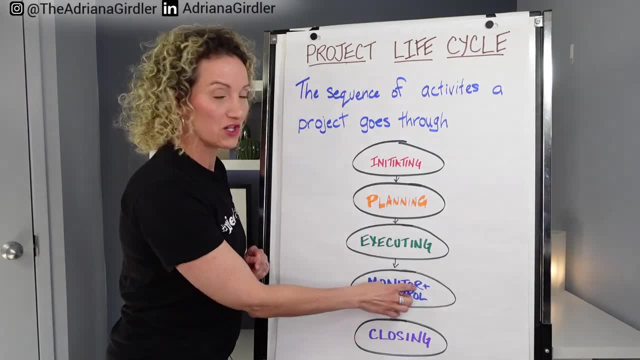 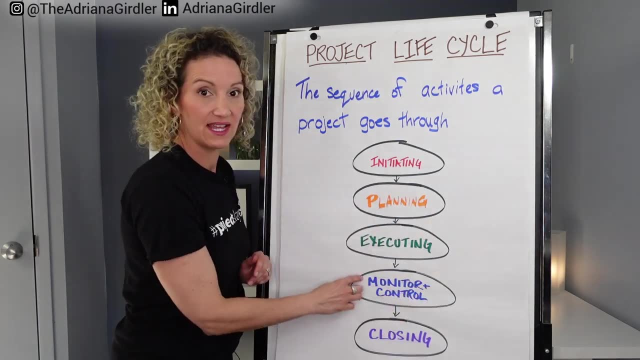 iteration that happens here. So you go, you're planning, executing, you monitor, control and then you may find something changes. You have to tweak a plan, a timeline, and it just goes through over and over This whole cyclical aspect of planning, execution and control. 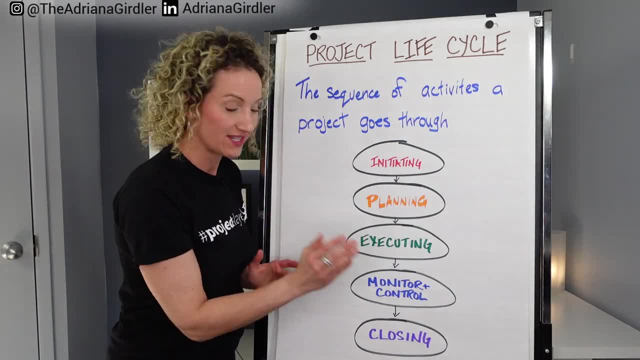 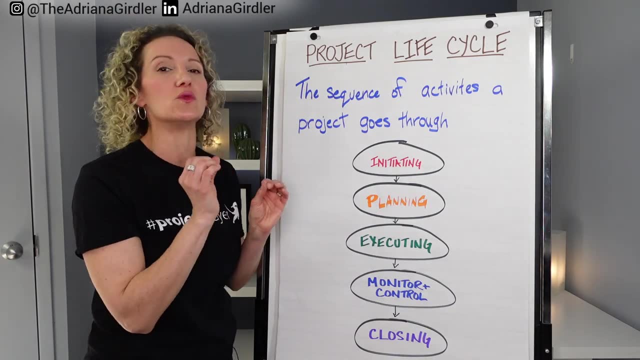 sorry, execution monitoring control, and then you execute it, And then you execute it, And then you go over and over until you get to the actual end. Now, people do forget about the end and they don't close things out properly. So, in order to really do well in project management, understand the 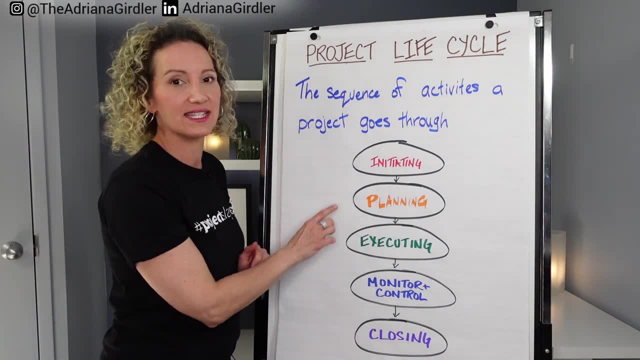 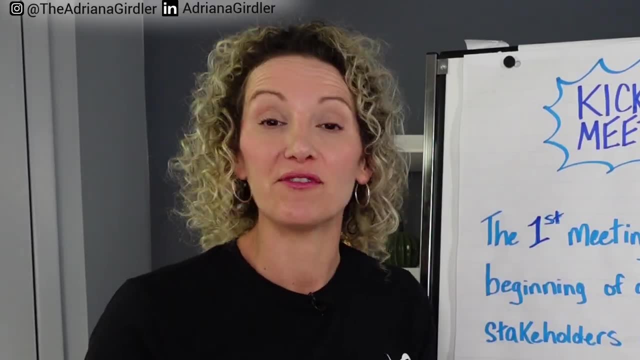 project life cycle, understand the stages and with every stage or specific tasks that you do, and it's something that I recommend you get to know really well. Okay, Before I get into this definition, don't forget to stick around to the end. 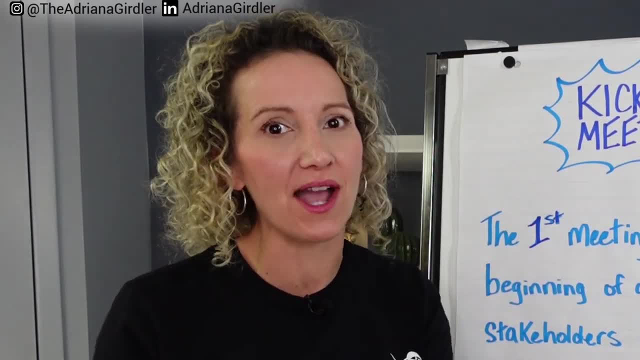 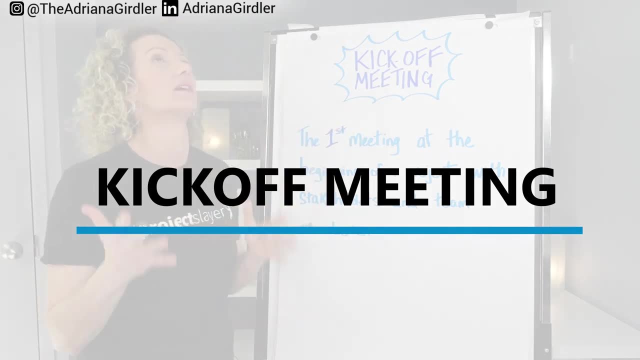 of this video where I'm going to share with you how to get your hands on my top 10 project mistakes checklist. You definitely have to stay in tune for that. Now let's go to this definition Kickoff meeting. Oh, this is a critical component of all projects is the 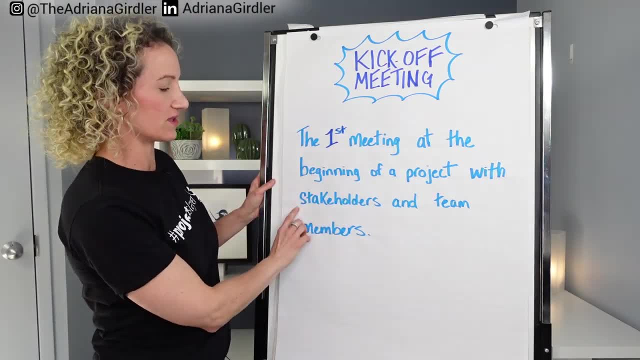 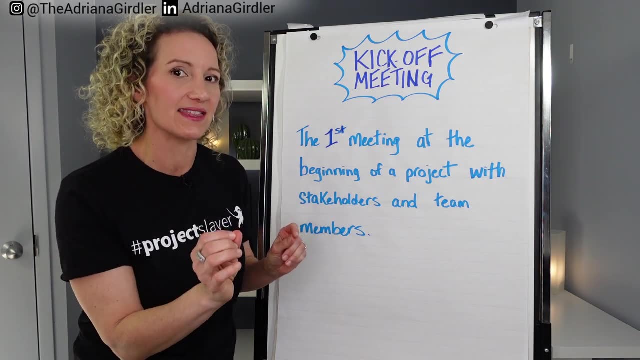 kickoff meeting. It's the first meeting at the beginning of a project with stakeholders and team members. Now what's really important is: your kickoff meeting is not the first thing that you do What, But it's the first meeting. Yes, it's the first meeting that you bring. 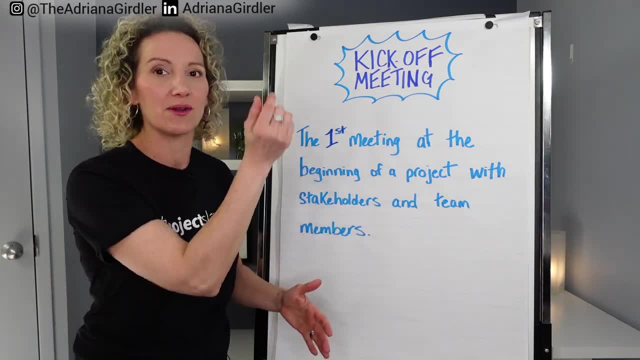 everyone together once you've done all your project, All right. So what we're going to do here is we're going to go to the first, we're going to go to the first three and you're going to go to the second: preparatory work. Remember, in the stages we said before, in planning this kickoff meeting happens. 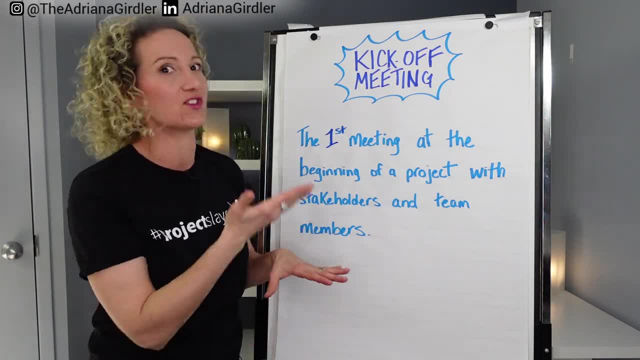 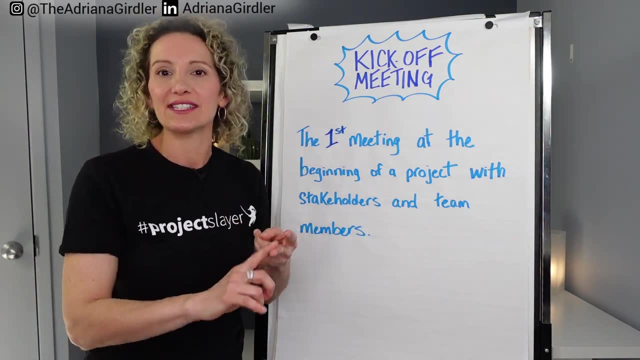 at the end of planning, right before execution. So there's still a lot that you have to do. So in this kickoff meeting, what are you doing? You're confirming the charter that you created. You are setting up expectations. You're probably even doing a little bit of action planning with. 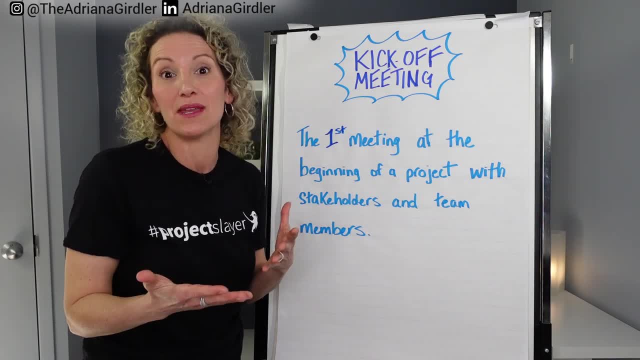 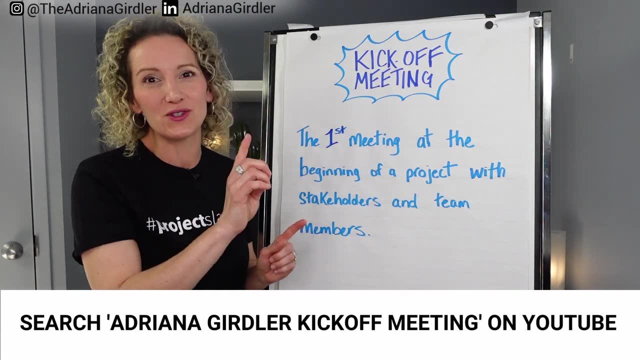 the team, because you're using your kickoff meeting really as a working session and maybe even a workshop. There's some really cool things that you can do. I got you covered, though, so if you want to know a little bit more about this, go to the YouTube search bar. Adriana Girdler- kickoff meetings. 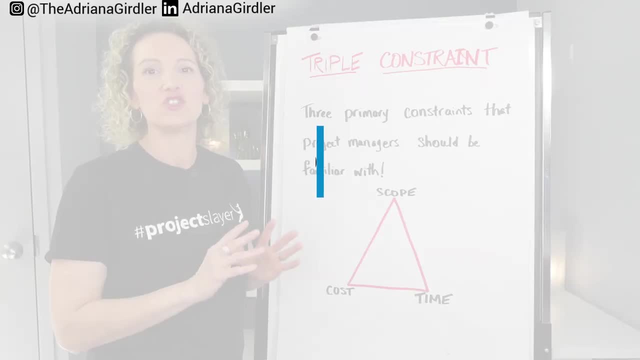 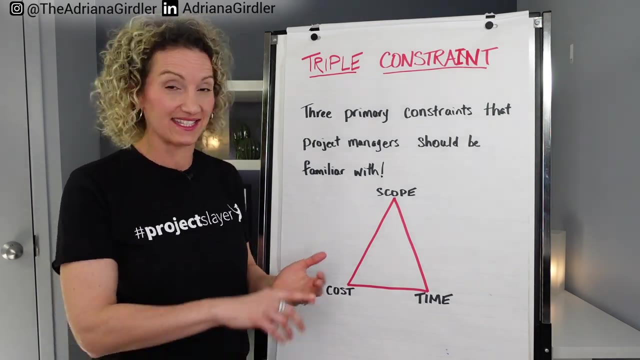 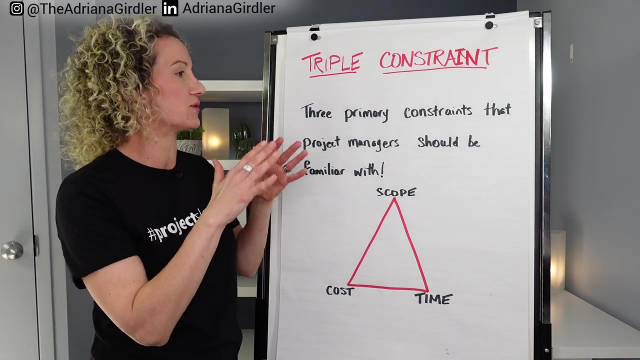 and there's a lot more great information that you can check out. Triple constraint, also known as the project management triangle or project priority matrix, because it takes some concepts of this, So let's get into this definition. It's the three primary constraints that all of us project managers have to abide by and should definitely be familiar with. 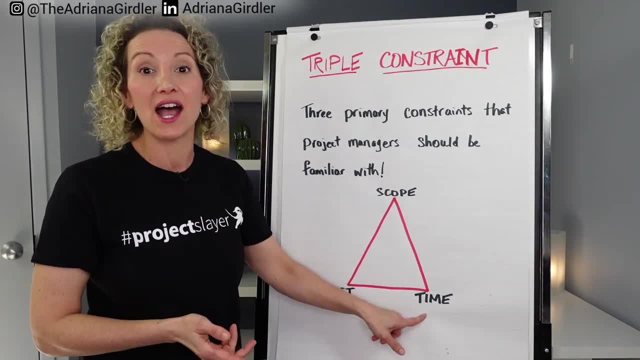 and that is scope. That is what is it that your project is doing. time- when are you going to be doing it? and time- time You're going to get it done in. and cost or budget- How much is it going to cost for you to? 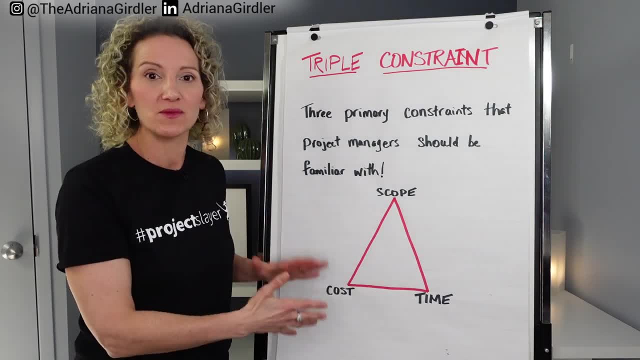 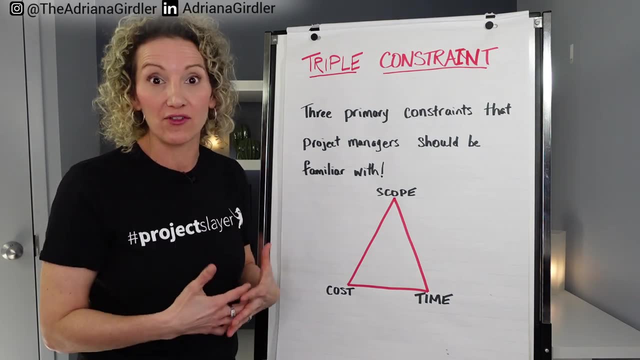 do all of this. This is what you're constantly managing As a project manager. if you want to very quickly say what does a project manager do? It's monitor and manage scope, time and budget. Whenever I talk to my team- and I try to course correct them- it's always about scope time. 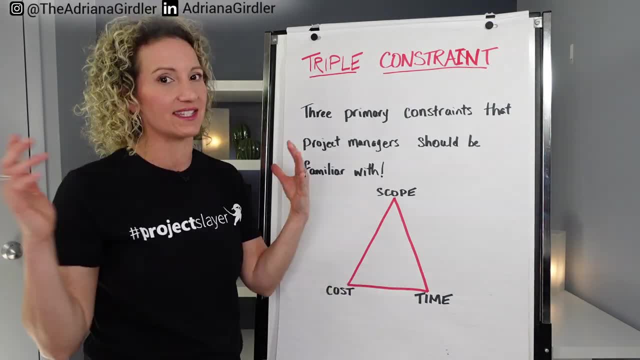 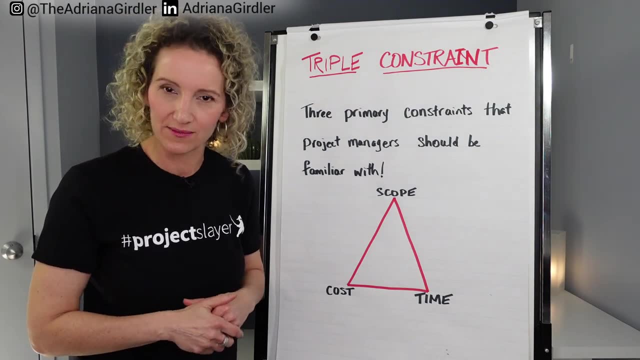 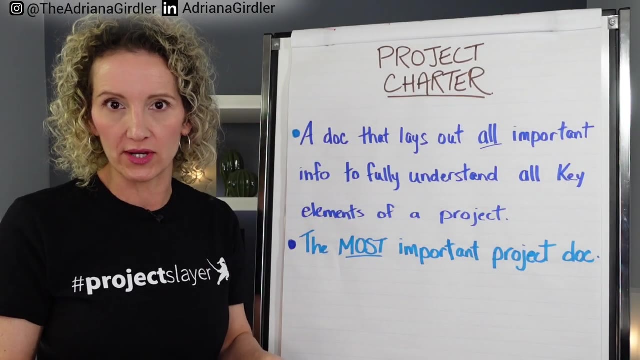 and budget. You don't want to oversee it. on scope, You don't want to exceed on time and you want to keep within your cost. This is what we're always trying to balance and it's known as that triple constraint Project charter. This is a critical, critical document all projects must have. In fact. 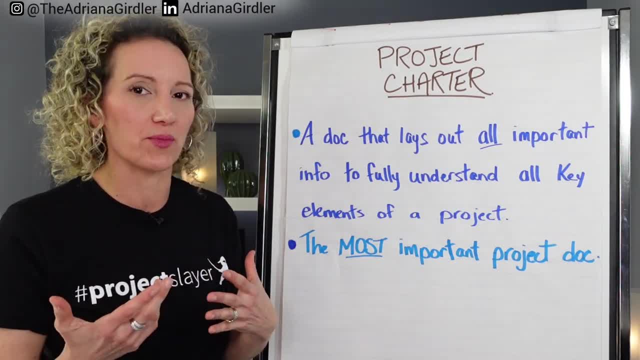 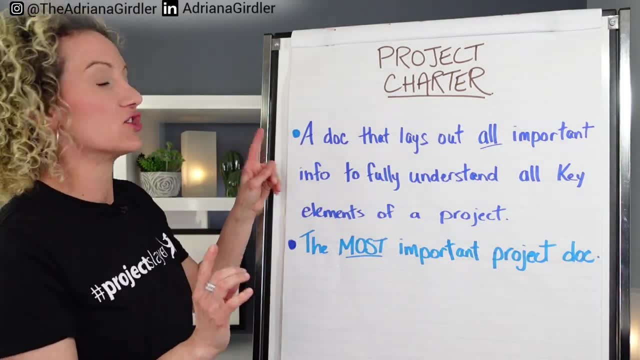 if you're asked to join a project or you're asked to provide input on a project, the first thing you should ask for is: can I see your project charter, please? Okay, so what exactly is it? It's a document that lays out all the important info to fully understand all key elements of the project. 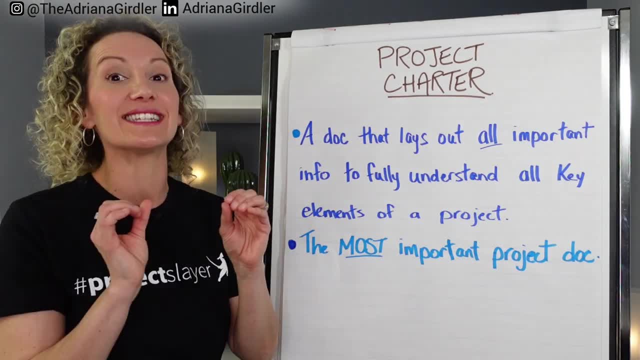 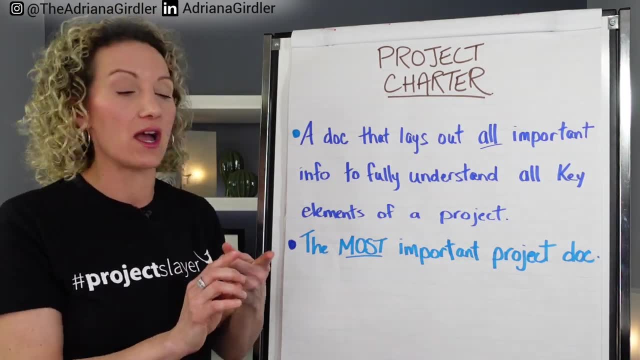 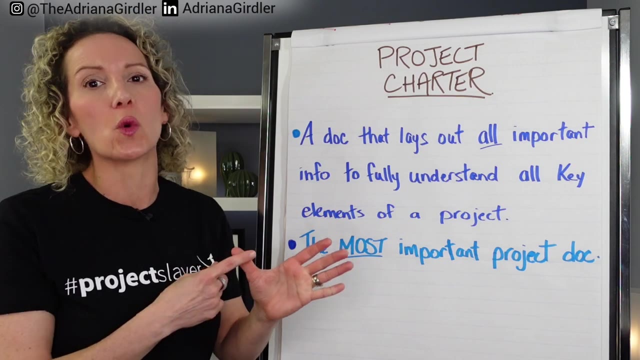 As I said, it's the most important project document, particularly during initiation and planning stages. What goes into this document? Everything from the scope statement to what's in and out, to high-level milestones, to priority project matrix, roles and responsibilities. 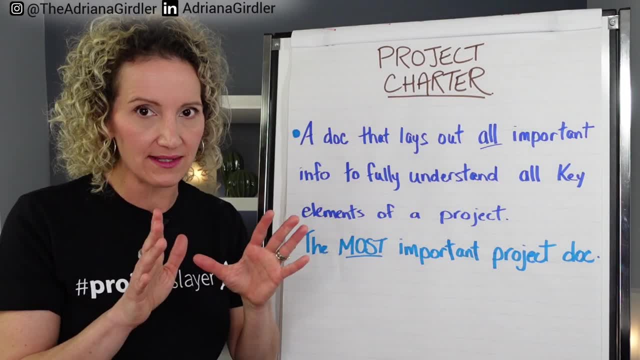 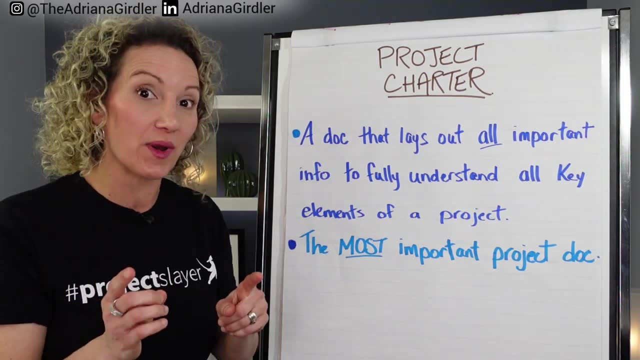 who's on your team. major milestones- Not detailed timelines, but major milestones- Anything that's going to help people who are joining your project, which, by the way, you're going to use this charter at your kickoff meeting. You're going to introduce it to everybody. 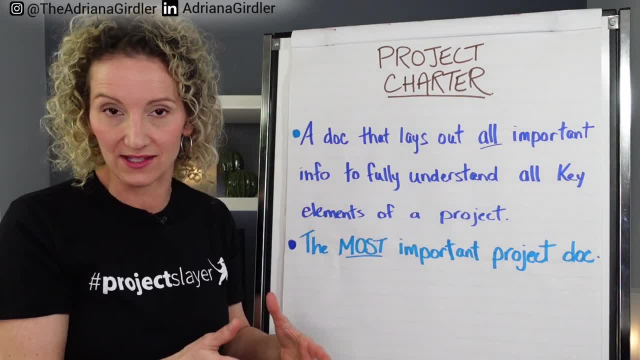 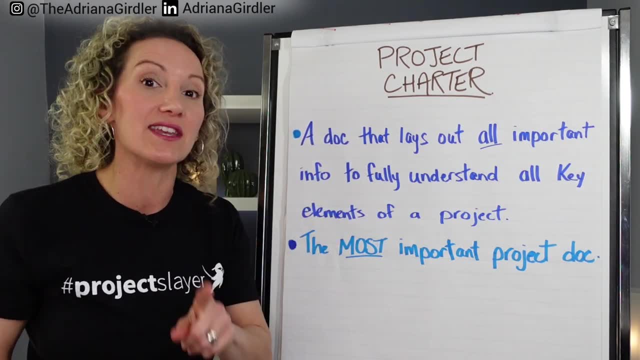 and you're going to give them a little bit of a sense of what's expected for them. You want the deliverable in that as well. This document is gold. I cannot tell you how critical it is to have this document. Now speaking of gold. if you're loving what you're hearing, please give this video. 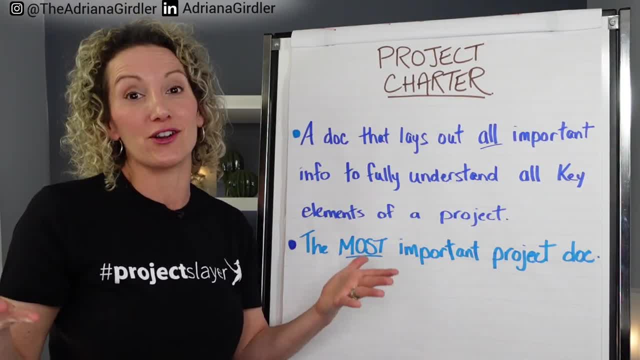 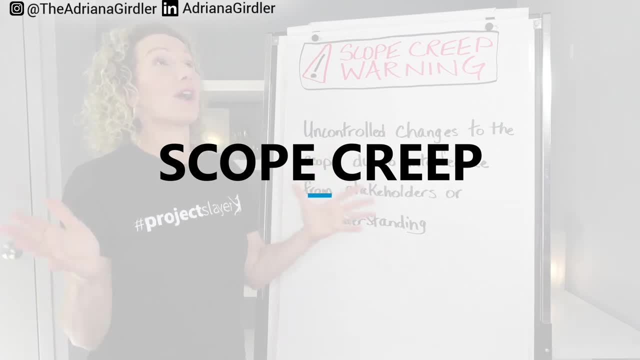 a thumbs up. It tells YouTube we're doing a good job, which spreads our channel and messaging to more people like yourself, So I'd appreciate that, Thank you. Scope creep: Warning, warning, warning, warning, warning. Do not do scope creep. Okay, What is scope creep? Let's talk about it. 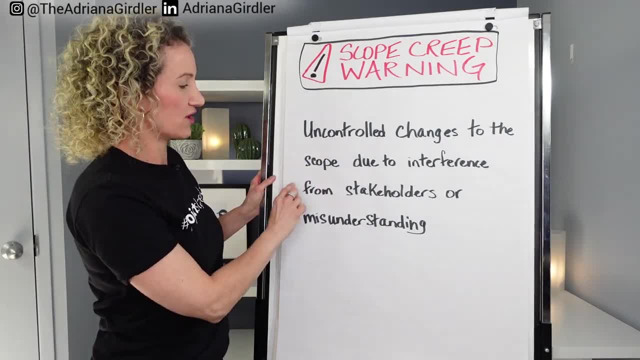 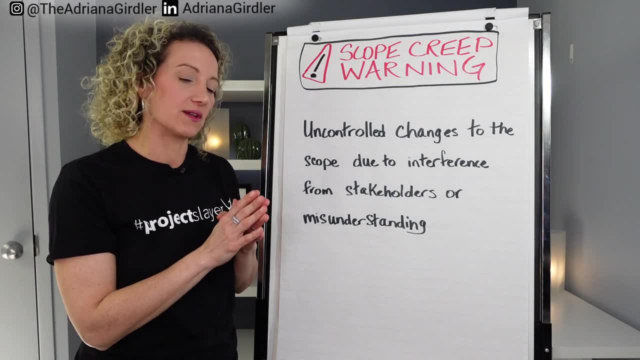 It's uncontrolled changes to the scope due to interference from stakeholders or through misunderstandings. Whoa, I bet you, once we talk about this, you'll go. oh, my goodness, you know how many projects had scope creep. This is where you have people outside. 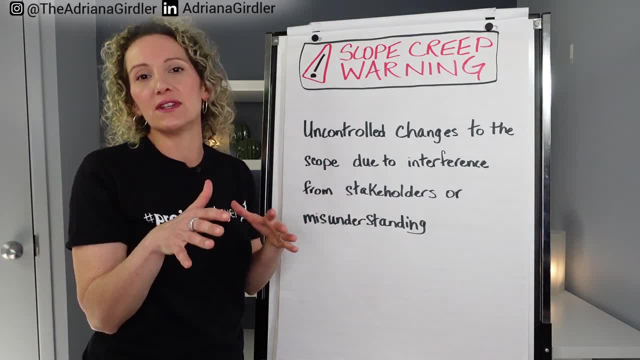 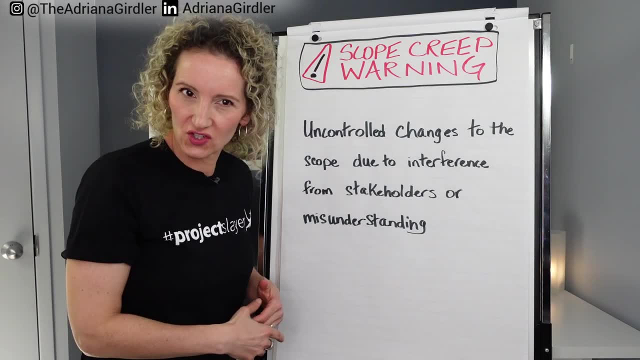 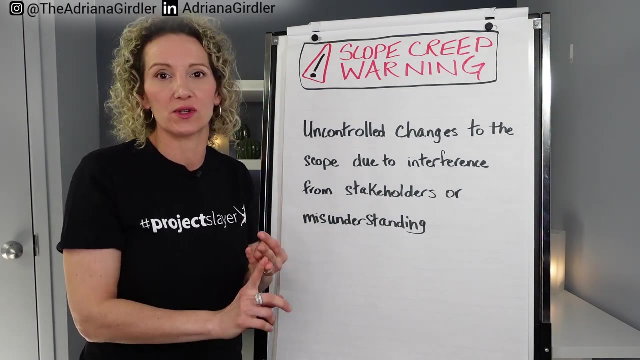 of the project who don't understand the details and are not privy to the project plan. Or it could even be senior executives, people who say, oh, just add this one thing to it And they want to expand scope, but they don't want to give you extra time or more budget or additional resources. 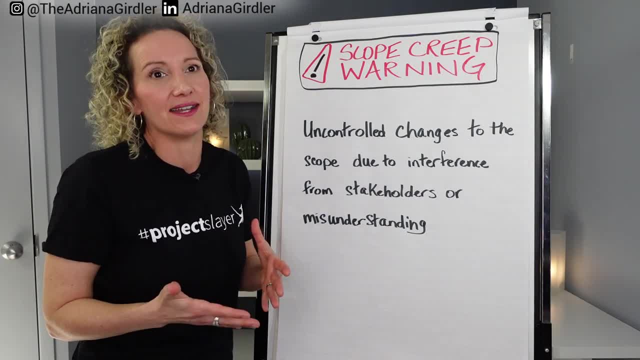 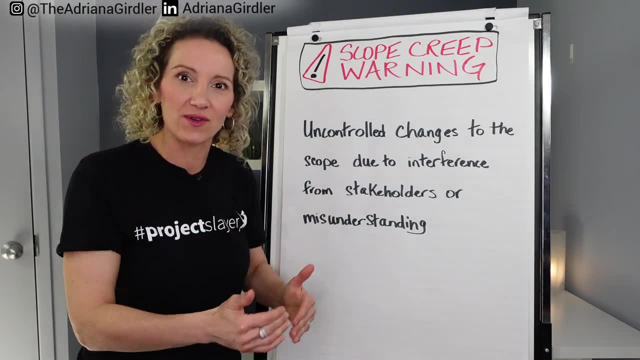 Because in their mind's eye it's super easy. It's not, And it's your job as a project manager to make sure you do not have scope creep. That's why you did the charter earlier on, to get everyone signed off on the expectations of what the scope was. 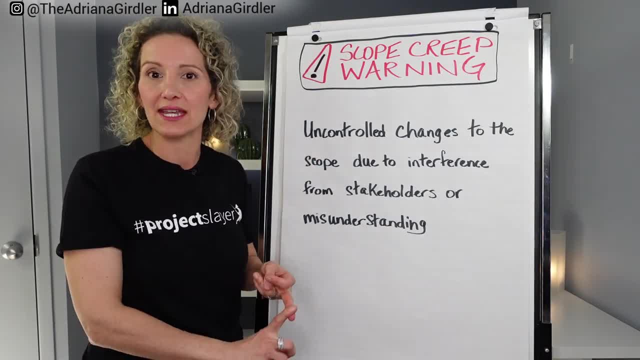 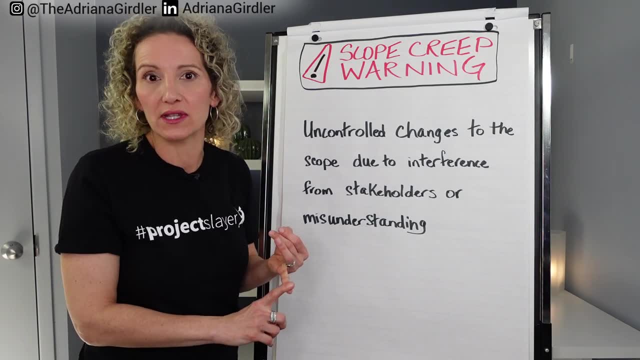 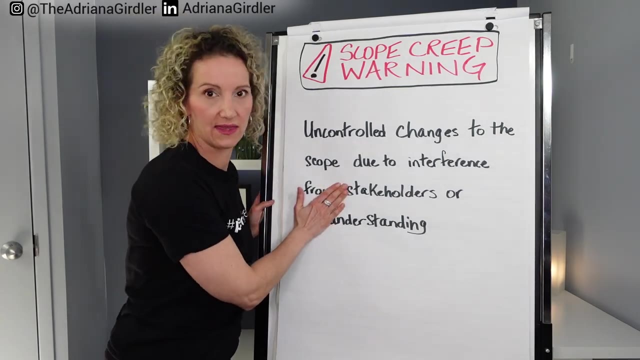 But scope creep will kill projects, It will lead to misunderstandings, It can lead to lots of assumptions And then it really at the end of people not being happy with the deliverable because there was scope creep. they didn't understand things. So really, warning: do not let this. 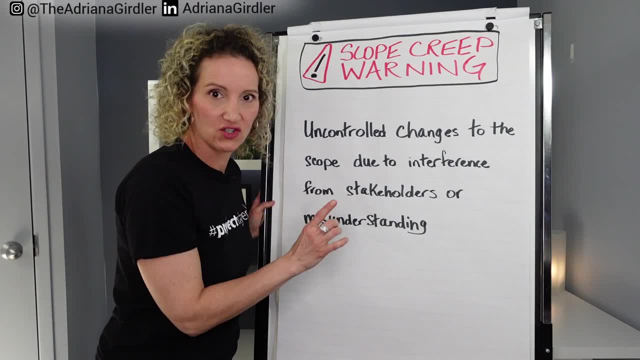 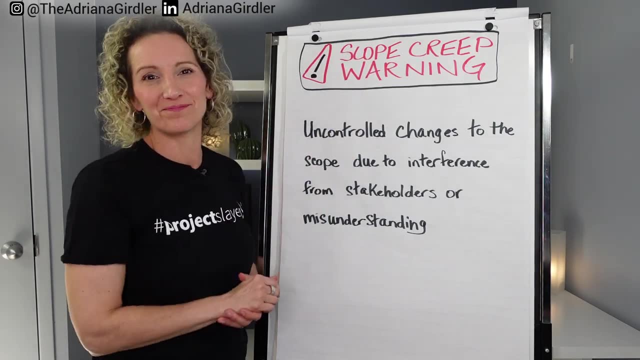 happen. Now what you can do, as I said before, have it in the charter, have everyone sign off on that document that I defined before and that's going to help you stop scope creep. Just be aware of it. WBS or work breakdown structure. Now, if you have heard or seen any of 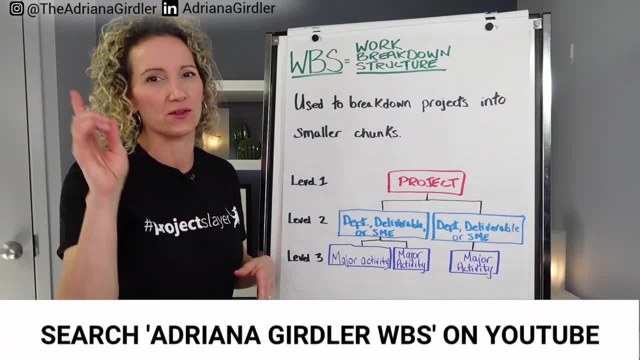 my videos. I do talk about the WBS. I actually have a really cool video. If you go to YouTube search bar Adriana Girdler and search work breakdown structure or WBS, it will pop up to give you a lot more information. 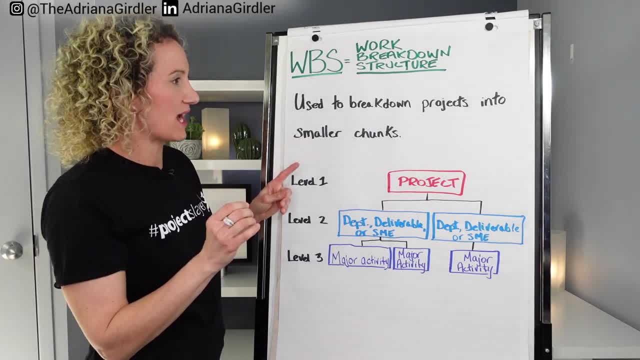 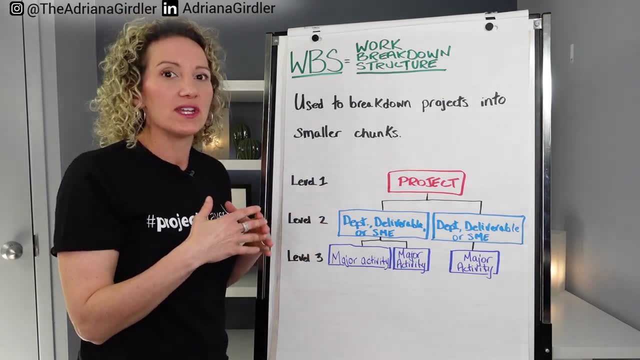 But I want to share with you the definition. It's used to break down projects into smaller chunks. So it's actually a technique that we, as project managers, use. When you're given a scope statement and you have this large deliverable, it can be slightly overwhelming. So the technique we 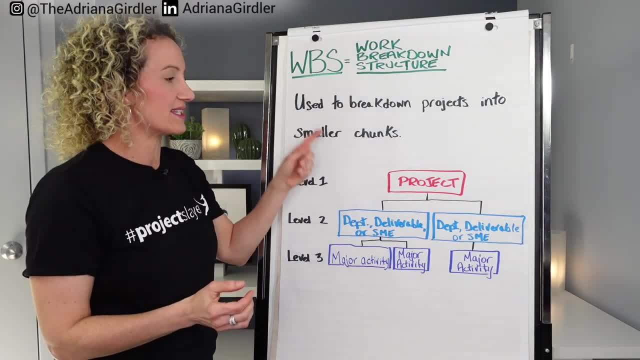 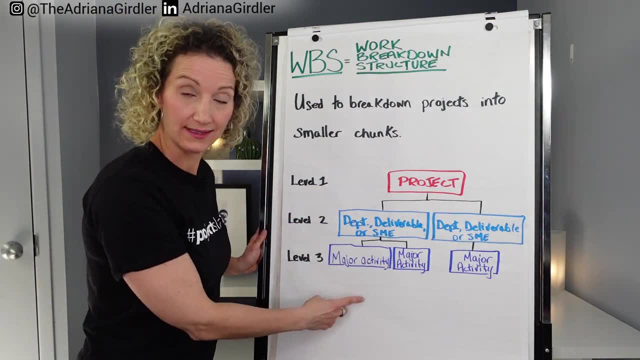 use is. we break it down. We do a work, breakdown structure into manageable chunks. So how does that look like? Well, it's kind of very similar to an org chart that you can kind of see here: Right, You start at the top, which is the project, Then that's your level one, Your level two. 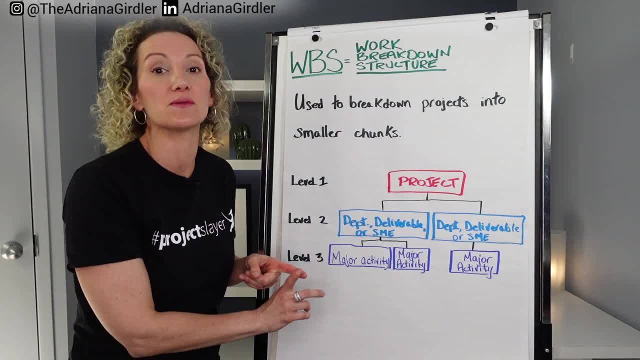 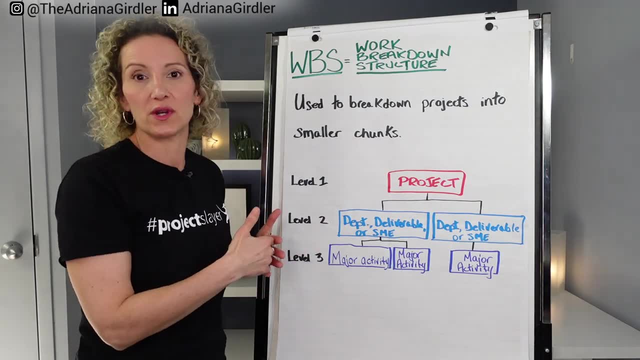 is. you then break things down either through deliverables- Maybe you have multiple deliverables. You want to break it down that way. Maybe you want to break it down by department- What does every department have to do? Or do you want to break it down through subject matter experts? 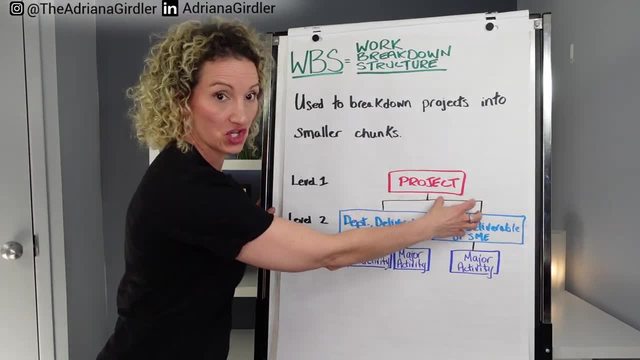 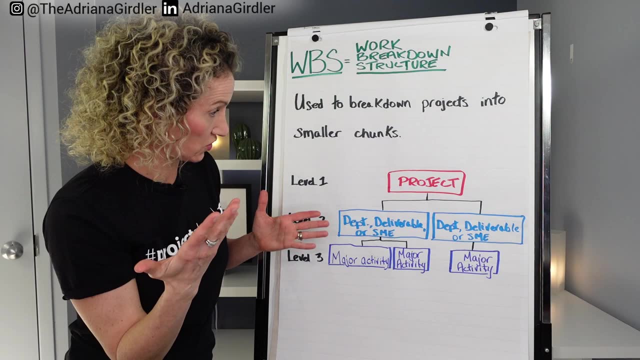 So you're breaking down into really more manageable chunks. Okay, So, for example, you may have a project of we have to install a new packaging line. Great, Perfect Project, Nothing wrong with that, All good. But that's a lot that you can do. So how would you? 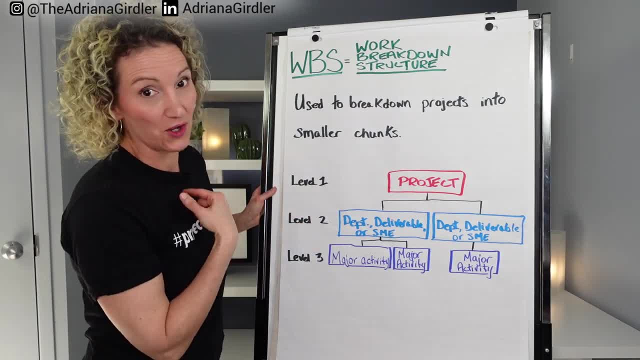 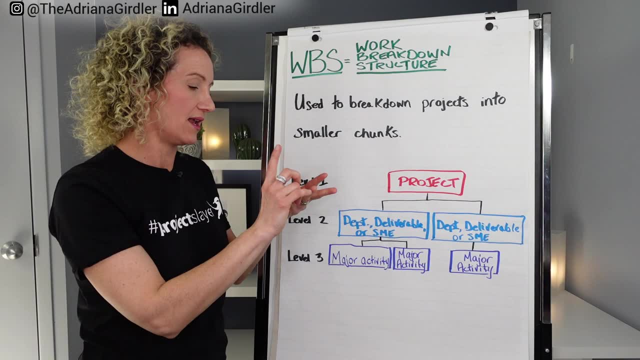 break it down into a level two. Well, I've done and installed packaging lines. So I have broke mine down through department because we had so many teams. I had a quality department, engineering department, We had training department, we had a production. So you, 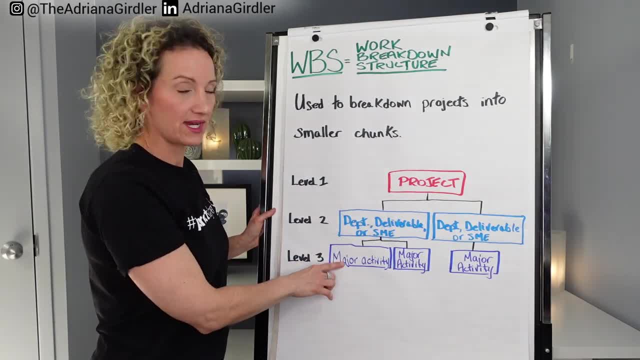 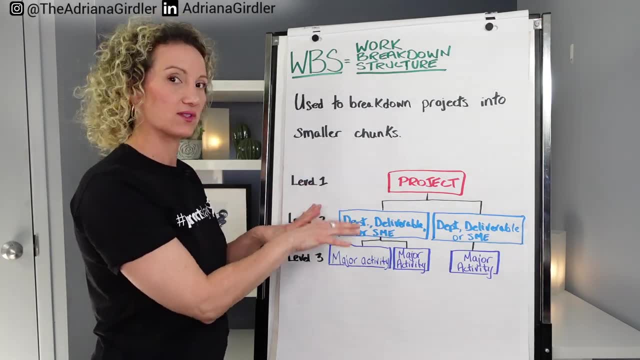 break it down And then, once you do that, you go okay. level three is for that big bucket. What are the major activities that have to occur? Because this is now where everyone's sort of getting into their role and responsibility. So, for example, if I had 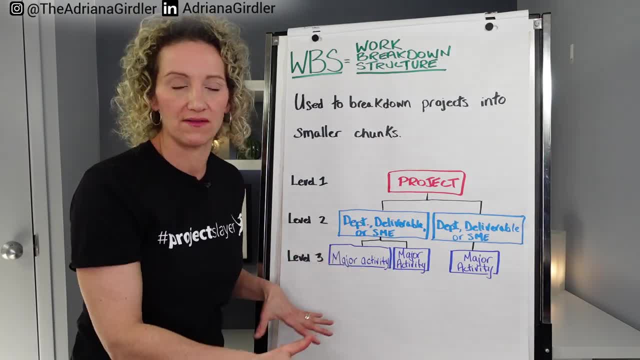 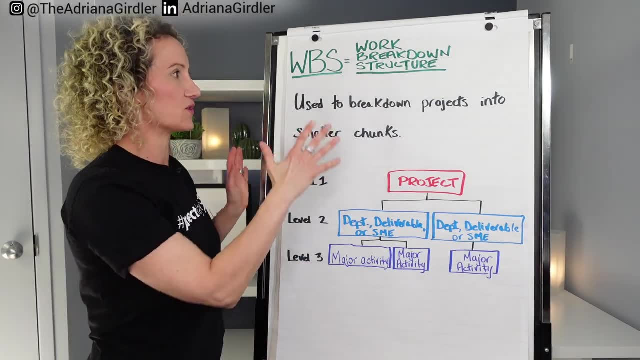 engineering. they would start breaking down all the major activities: purchasing of the equipment, testing of the equipment, writing up of the documentations- like they're really getting into that level. So now you have a really easy way, and very quickly, of understanding. 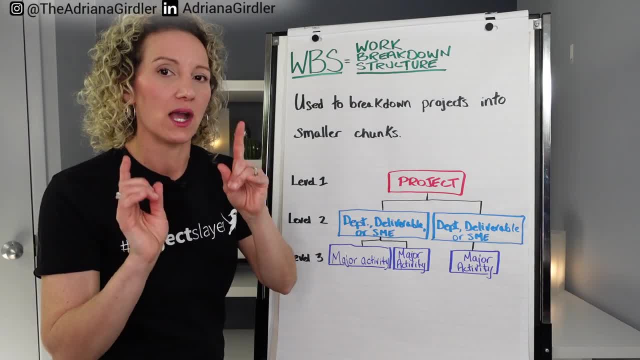 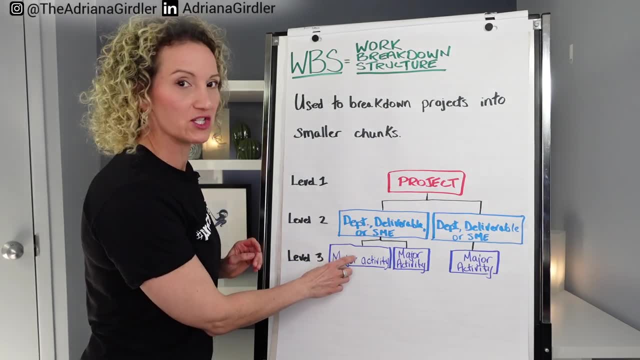 what your project's all about and what are all the moving parts. Now, what's really cool. This is a little bit of a bonus for you. Bonus tip: You could do a level four, and that level four is with all the major activities. You can break down those major activities into detailed tasks and 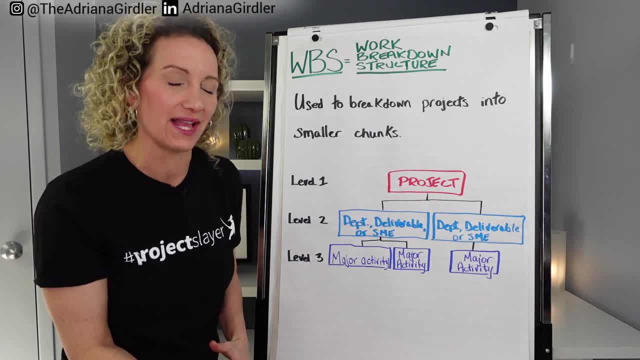 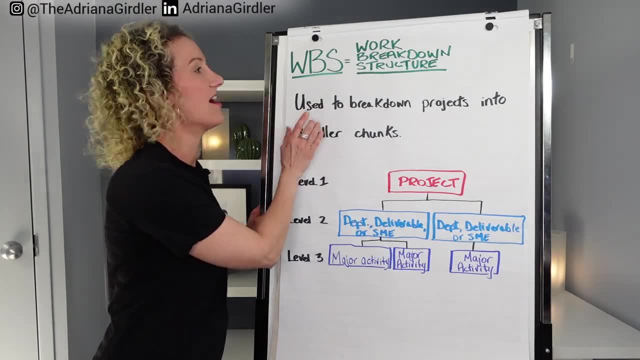 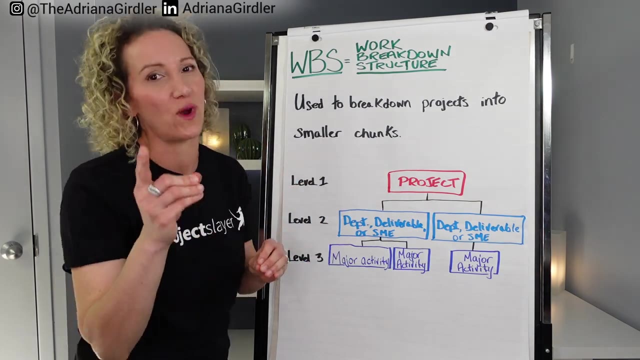 then use your WBS as an action plan. In fact, that's what I do I use. I call my action plan a WBS because I base it off of this- It's really a springboard- off of this technique of breaking down projects into manageable chunks so that you can successfully know what you have to execute. 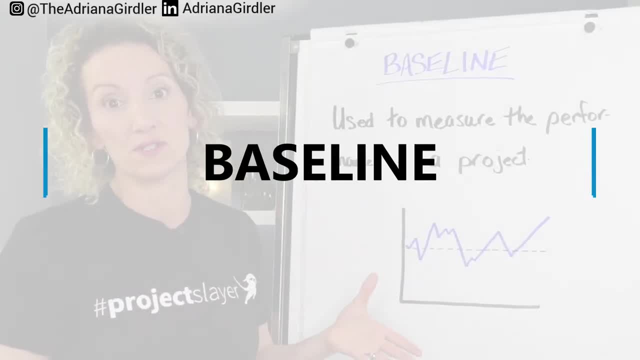 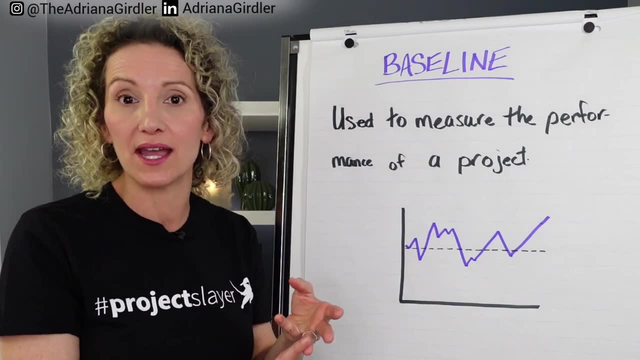 Baseline. This is a very common terminology used amongst project managers. You're baselining your original plan, which is around your scope, your project plan timelines, budget, So you're using it to measure the performance of your project Now. 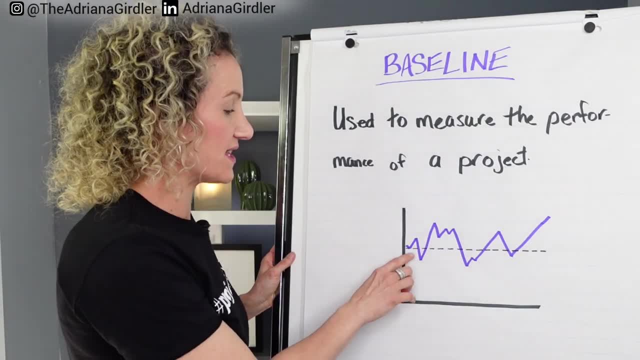 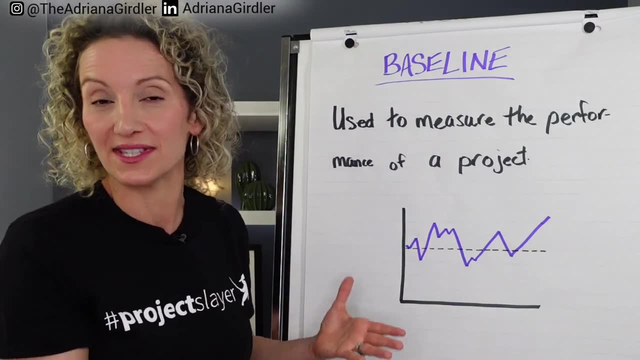 for example, with this one, this could be a budget baseline. So if this is what my baseline is and that's what you agree to, you can see all the ups and downs you're monitoring through your project management tools and techniques. But again, you have baselines for practically that. 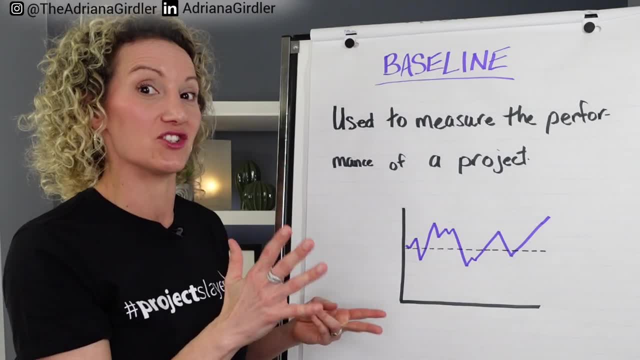 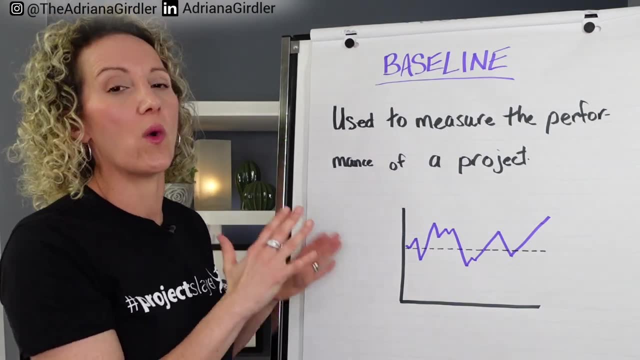 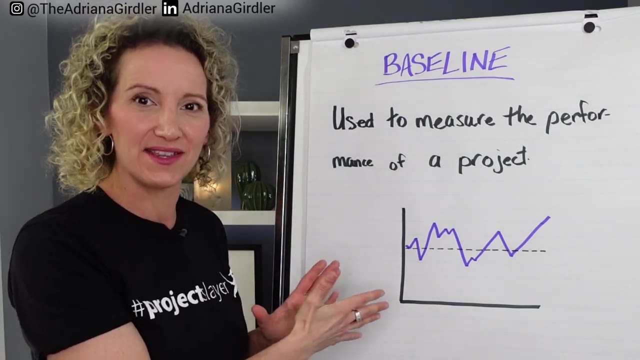 triangle that we showed you. Remember the scope baseline. has anything changed? Timeline baseline, budget baseline- It just really ensures a nice way to know: are you on track, not on track, What deviated? So in the future if you have a similar project you would refer back to your original baseline that you did. 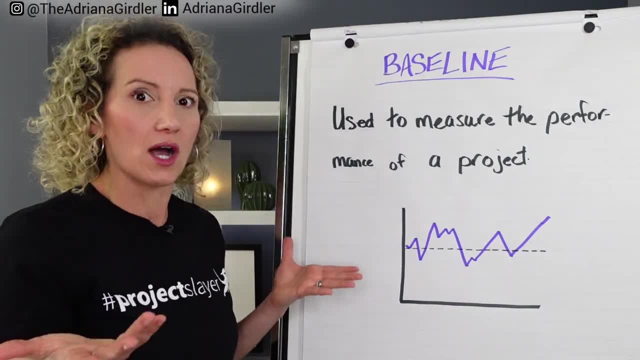 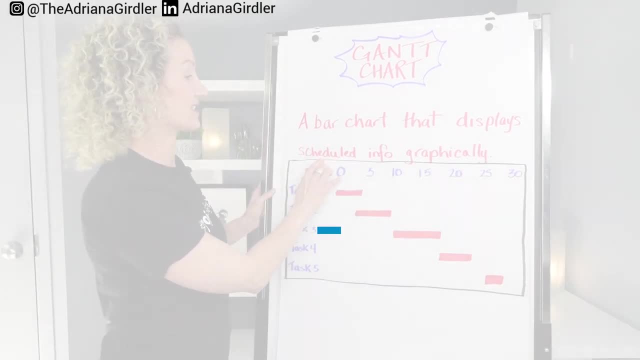 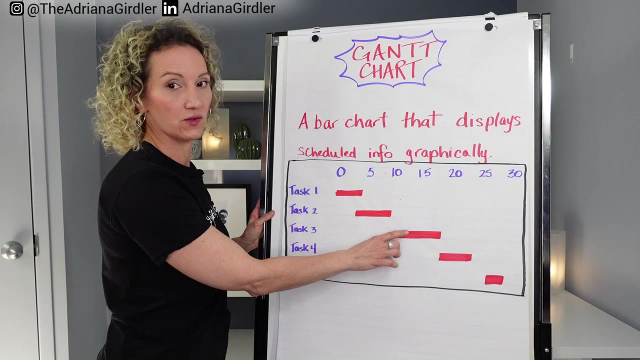 in another project to see what you can learn from it. It's a very good common technique we use as project managers Gantt chart. All right, A Gantt chart is a bar chart that displays scheduled info on your project. So you can see that, right. You have what your tasks are. you have your timeline. 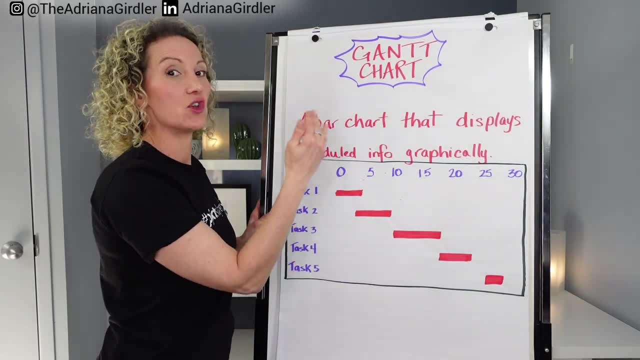 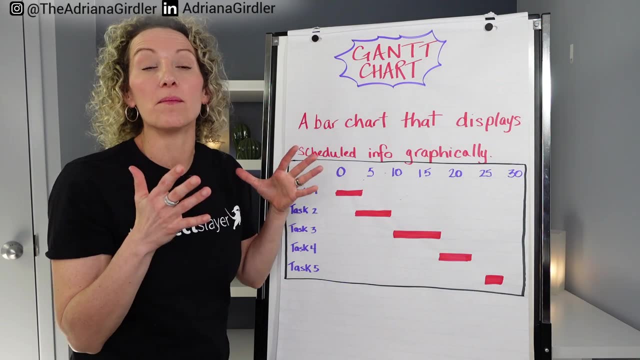 there and it shows you through a bar chart what exactly things are going to be done, And if you go a step further, you could even do dependencies, et cetera. Now I really want to be clear. It's a great tool for monitoring your timeline, to understand dependencies or what flows into a 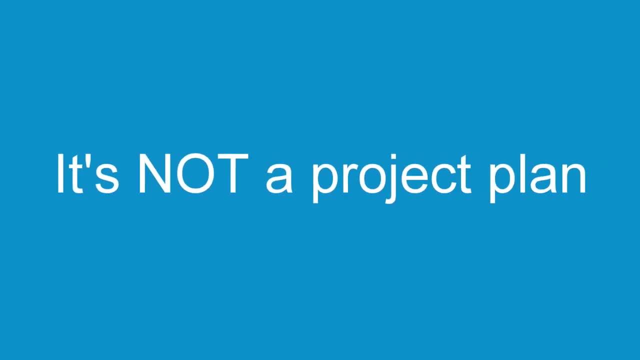 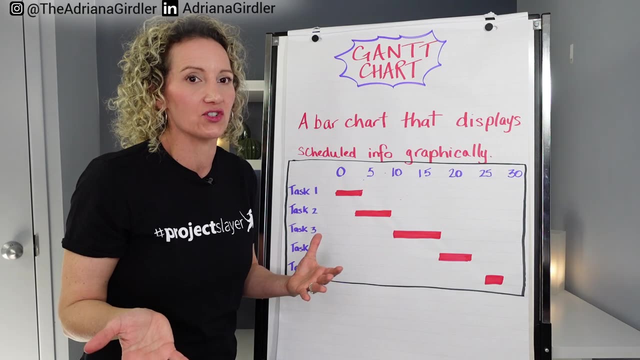 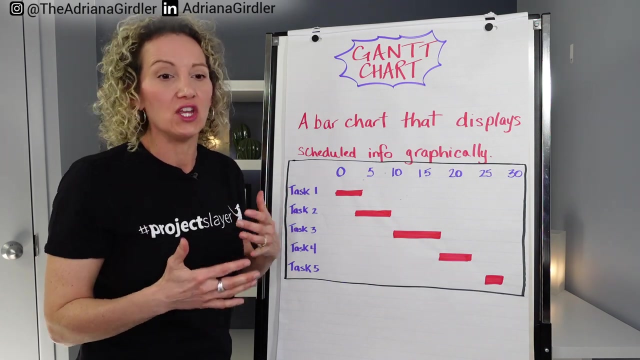 task or out of a task. It is not a project plan. Please do not have only a Gantt chart. that is too often in projects And I'm letting you know you are missing out on a lot of other stuff that you need to be cognizant of. You actually need a detailed project plan that has 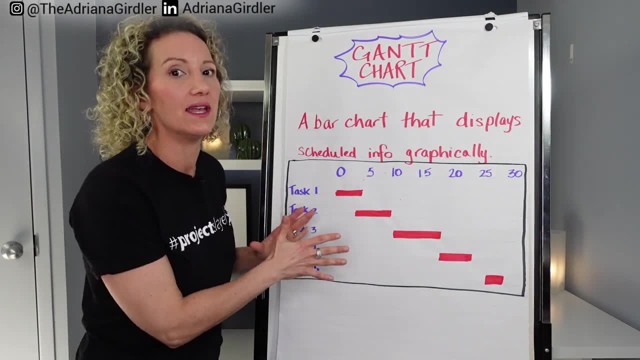 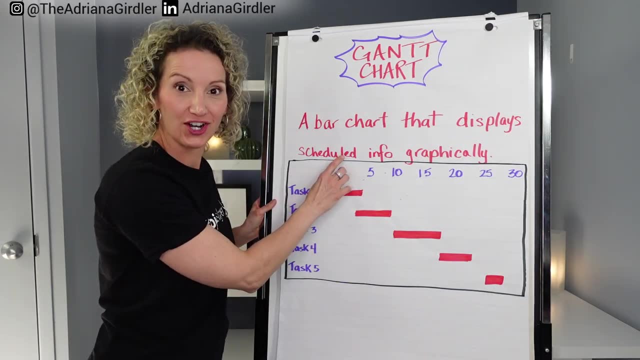 a list of tasks, et cetera. You can't do that with a Gantt. It's too overwhelming. I've seen Gantt charts which are humongous and people don't look at them. And the whole purpose of your Gantt chart. 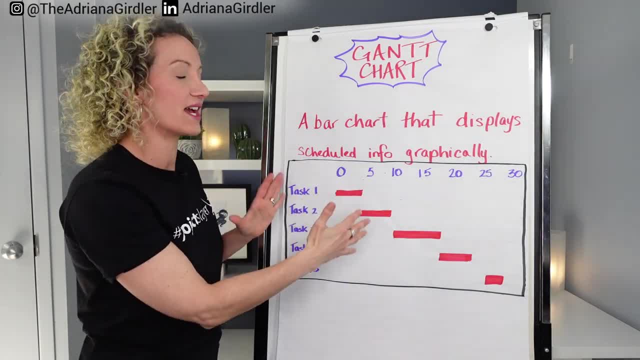 is, so you can see very quickly dependencies where things are at. are you on track? So it is a really good tool. It is for the timing, So I'm going to show you a Gantt chart that I've been using for a long time And I'm going to show 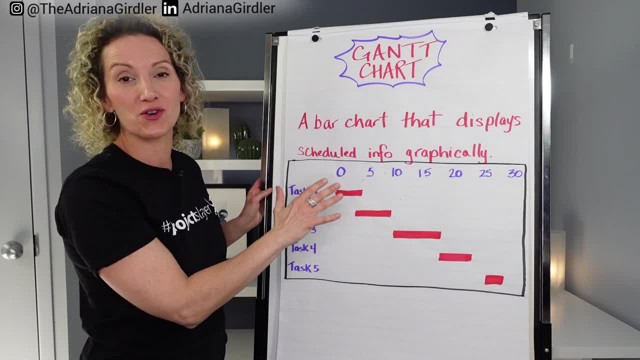 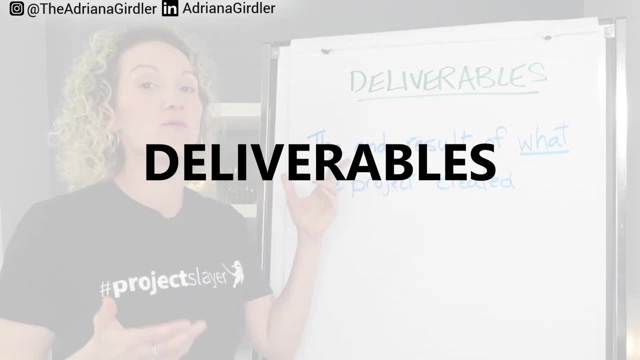 you the time portion of your project when you want to monitor the schedule. It is not a project plan. Just please remember that. Last but not least, deliverables. And what a great way to end on this terminology. Why? Because every project has deliverables. 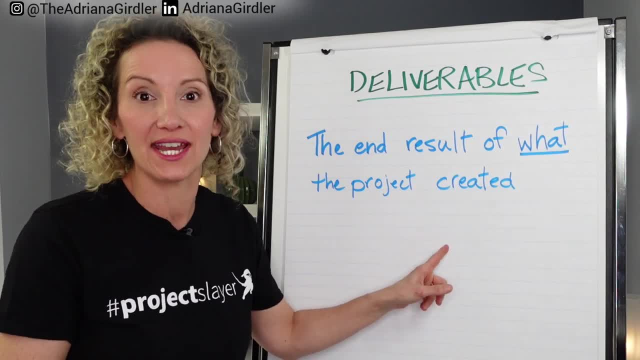 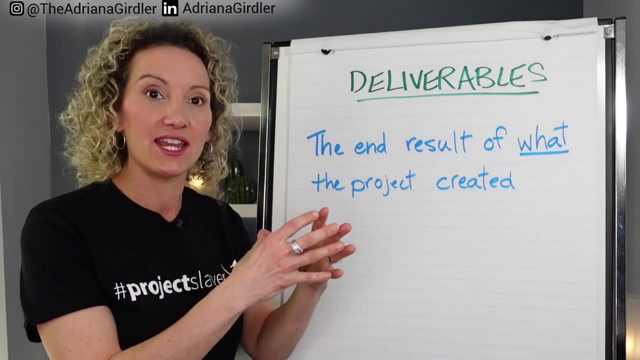 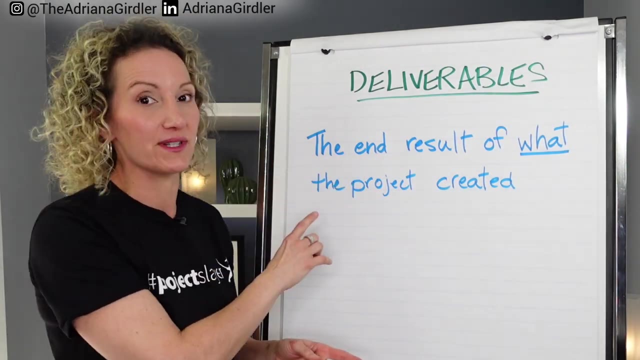 And what are deliverables? It's the end result of what the project created in order to give to a client, an end user, a department, whomever you were creating your project activities for- you're now delivering it to them. That's what a deliverable is. Now I have for you a deliverable. 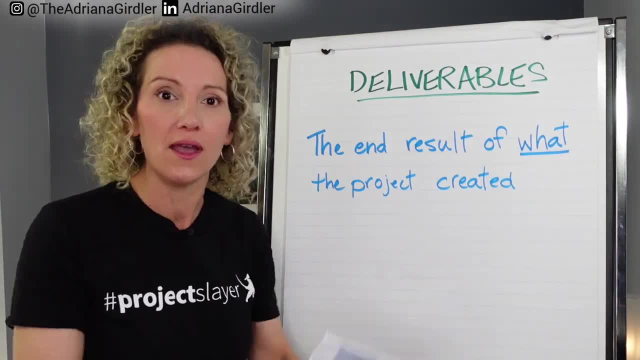 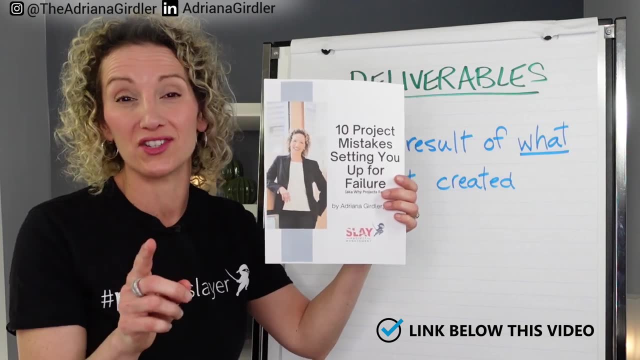 And that is I told you, if you stay to the end of this video, I was going to thank you by giving you this, free, free, this great checklist that tells you all the top 10 mistakes in projects. You're definitely going to need this, And how can you get it? Go to the link below this.